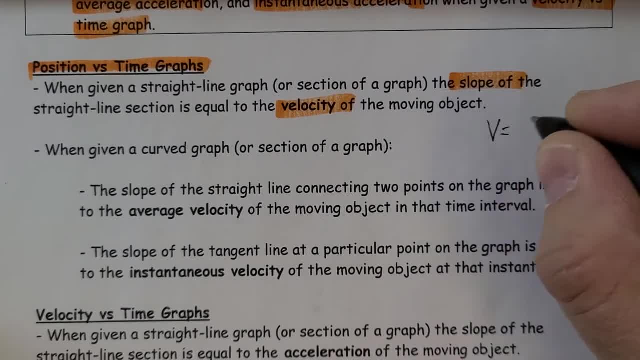 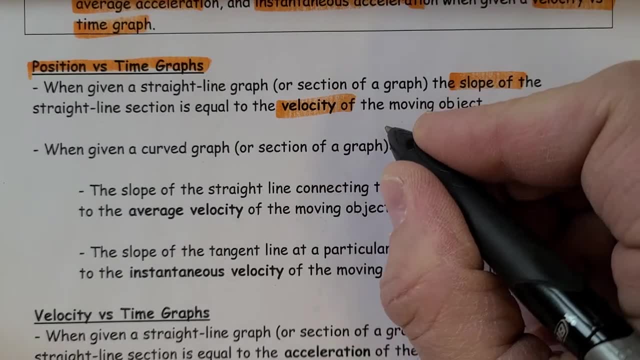 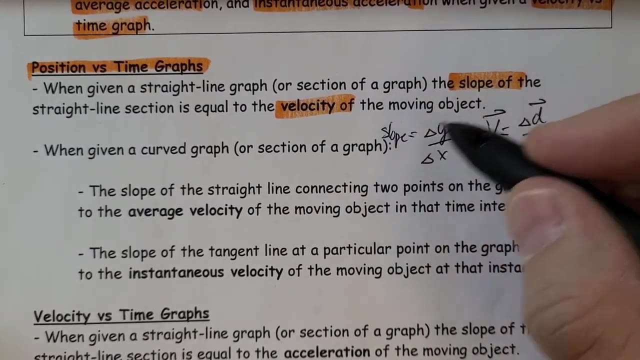 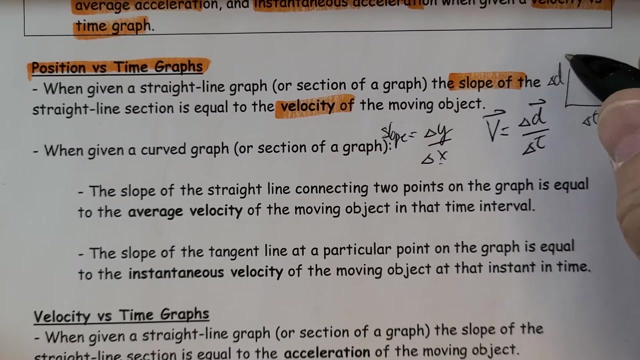 And you know what That makes sense? because the equation is delta D over delta T And, of course, where have you seen that before? Slope is equal to change, Change in Y over change in X. So rise over run, and on a velocity versus time, or sorry, a position versus time graph, our Y is represented by D and our X is represented by T. 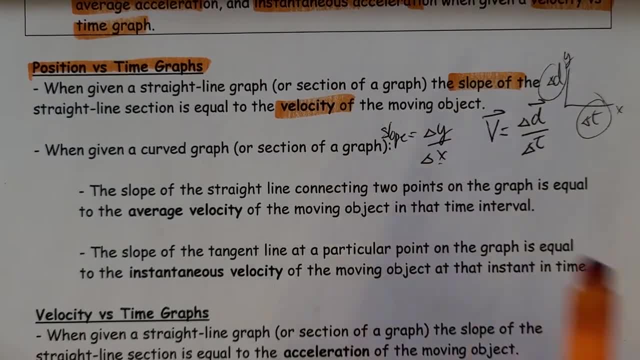 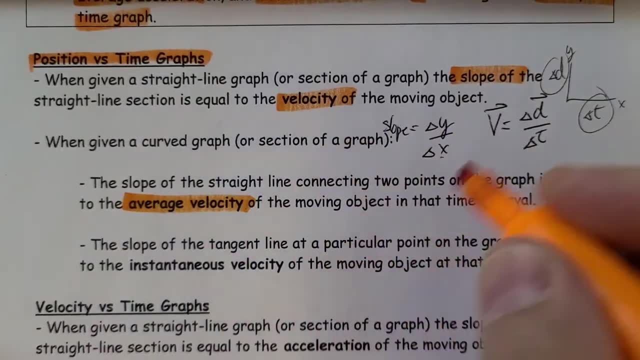 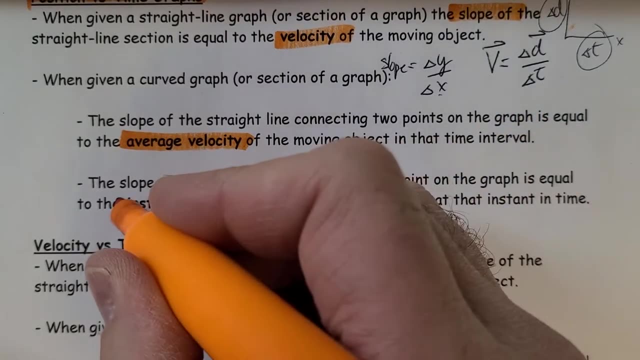 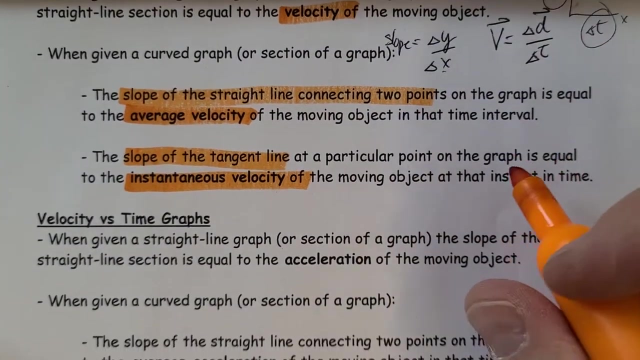 So if it's a straight line graph, the slope gives us velocity. If we're looking at a curve graph, the slope of a straight line connecting two points would give us average velocity. If it's not a straight line graph, And if I want the velocity at a particular instant in time, we're going to look at the slope of a tangent line, giving us instant velocity. 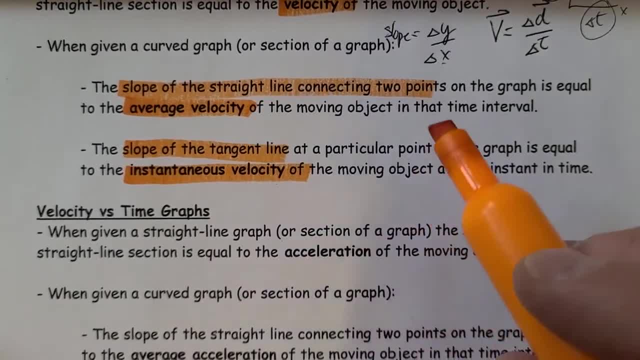 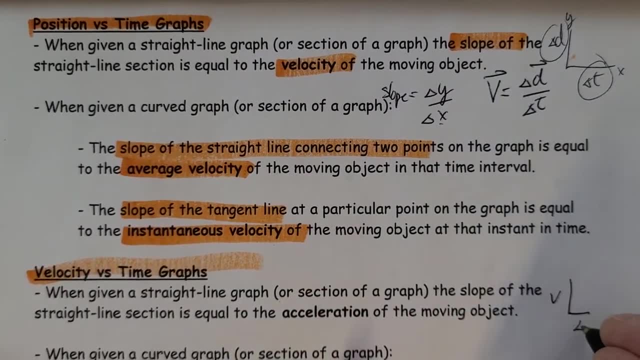 So it kind of is a peek at what you'll be doing in calculus. Now, if I look at velocity versus time graphs, guess what? It's very similar V versus T type graphs. And again, look at our: Y is represented by V. 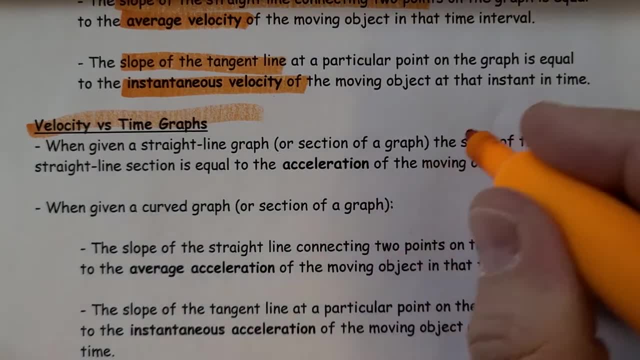 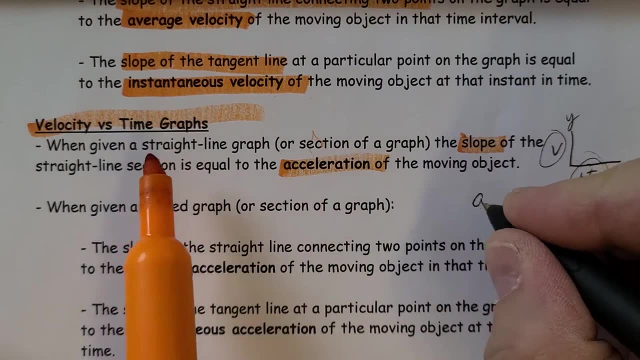 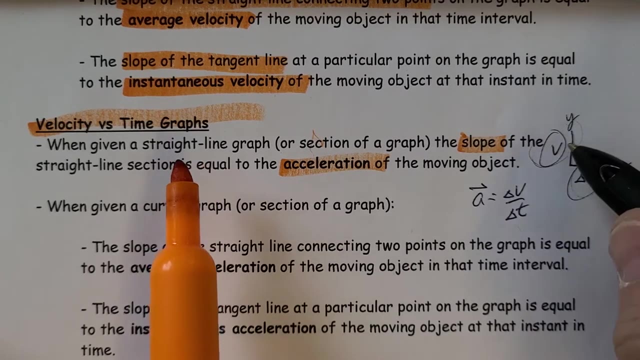 Our X axis It's represented by T. So again the slope of that graph gives us acceleration. And again that makes sense, Because acceleration is change in V over change in T, Change in Y over change in X, But in our particular case, change in V over change in T. 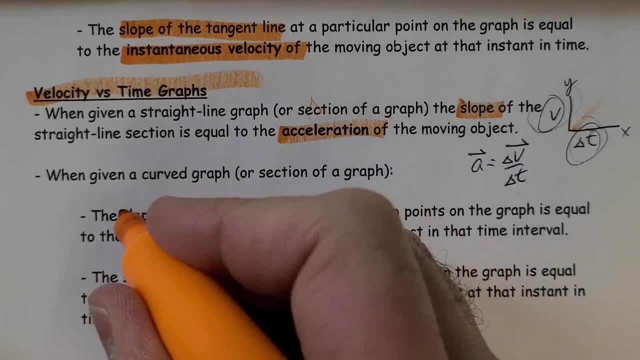 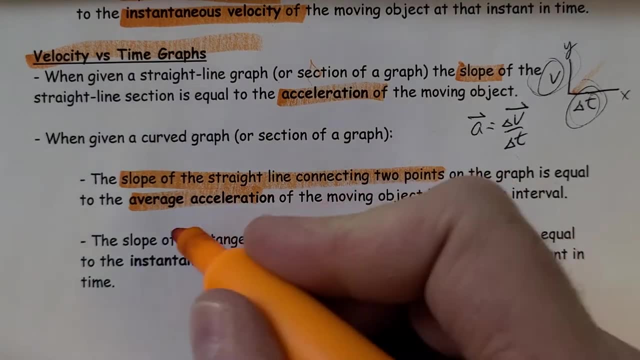 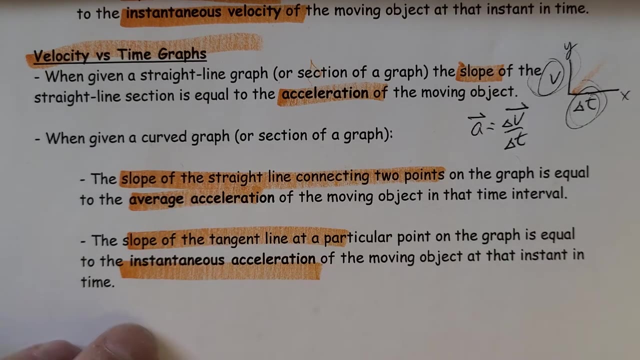 And of course, if it's not a straight line graph like that, the slope of a straight line joining two points would give us the average acceleration of that object in those two, And of course the slope of a tangent line at a particular point would give us instantaneous acceleration at that point. 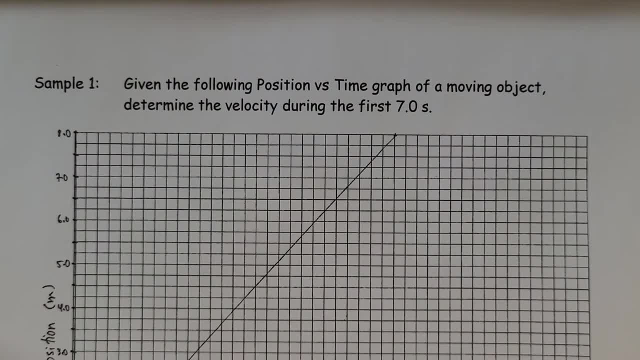 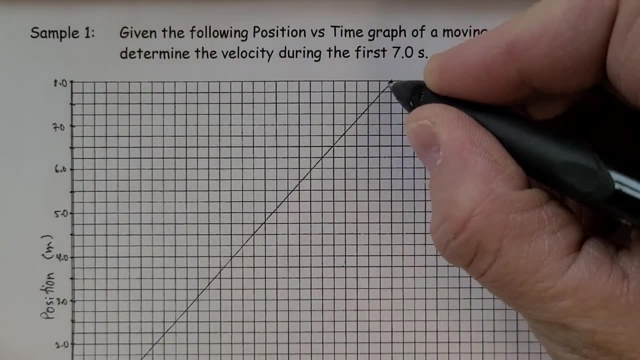 So we'll go through all of these scenarios. So, given the position versus time graph of a moving object, determine the velocity of the first seven seconds. So first seven seconds takes us up to here, Right, And it's a straight line graph. 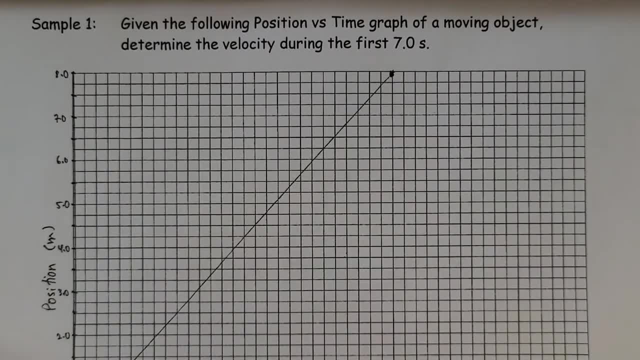 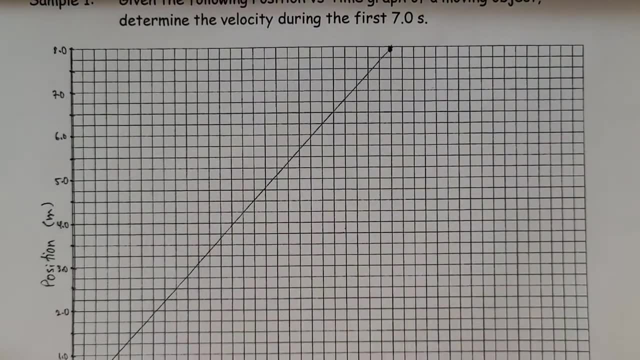 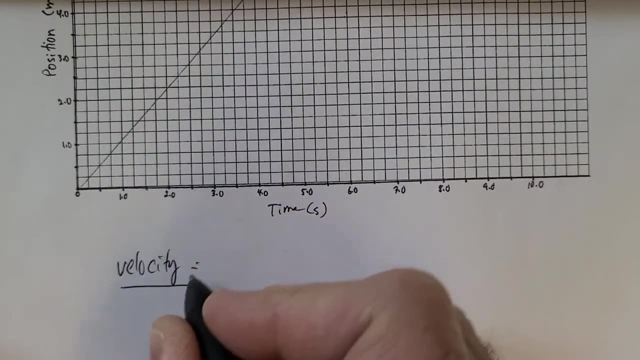 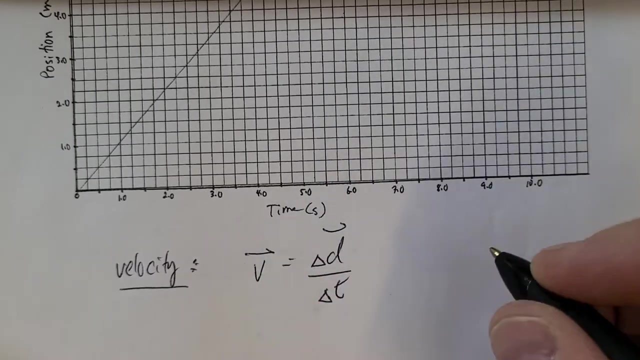 So if I'm looking at the slope or looking at velocity, it's just simply going to be a straight line And I can just simply call it velocity. So velocity is V is equal to change in D over change in T. Now, since I'm looking at the first seven seconds, I'm going to be looking at two points here. 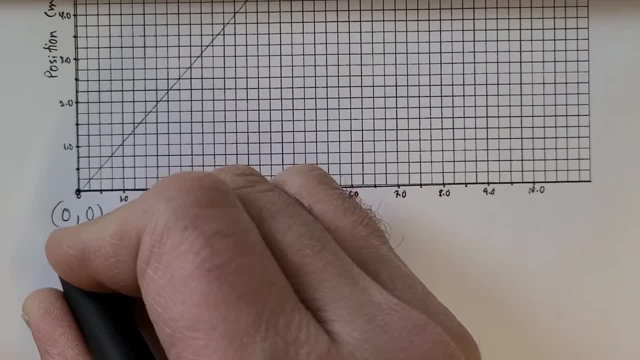 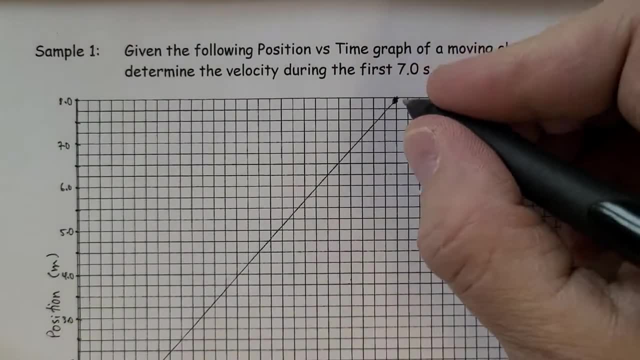 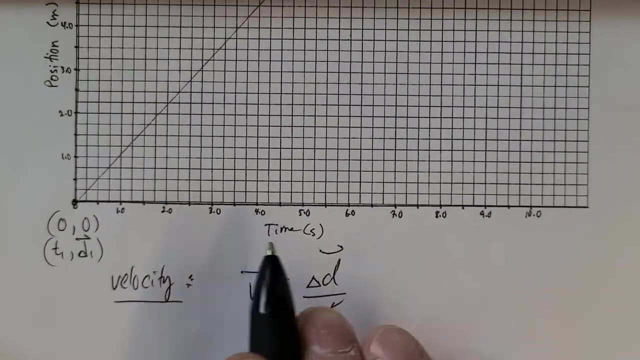 I'm going to be looking at 0, 0,, which is my T1.. So I am looking at a clock reading at 0 and 0.. Then over here, basically looking at the coordinate of a point right: X, Y, but in our case T, D. 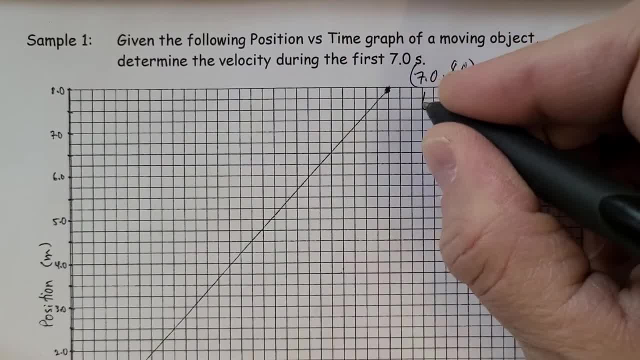 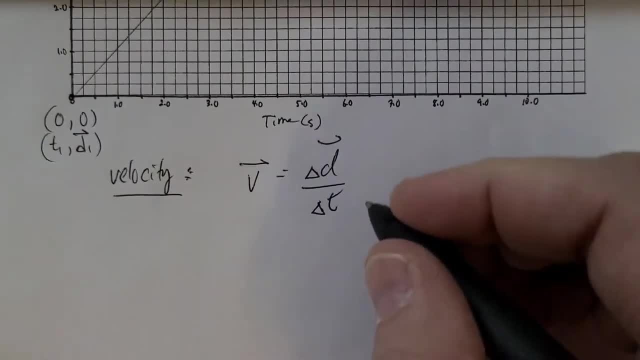 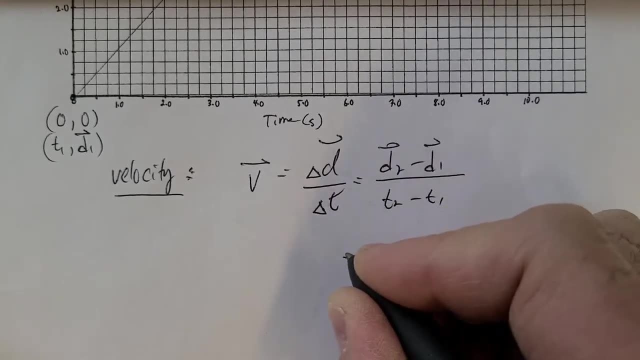 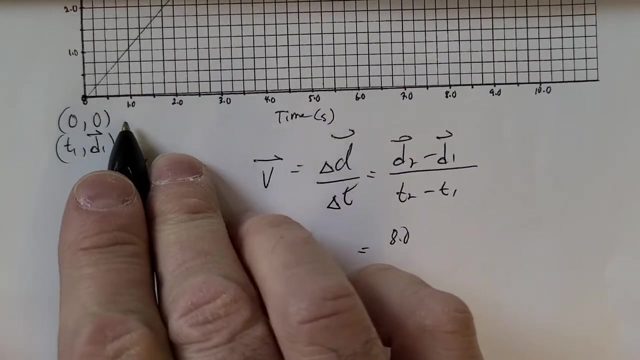 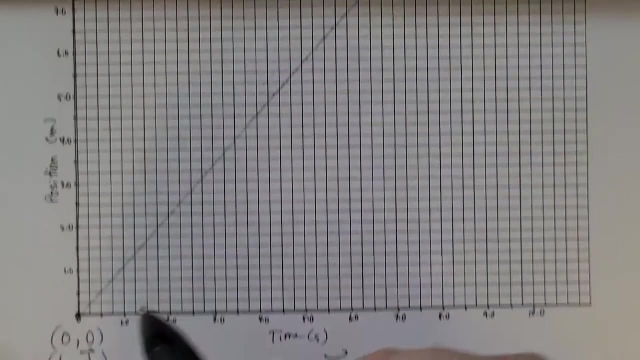 So this is at 8.. So that is my T2, D2 point. So over here, D2 minus D1.. Over T2 minus T1.. So my D here is 8.. My initial one was 0.. And then my T2 point is 7 minus 0. 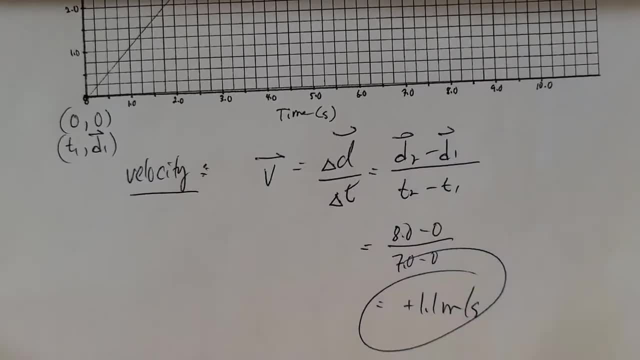 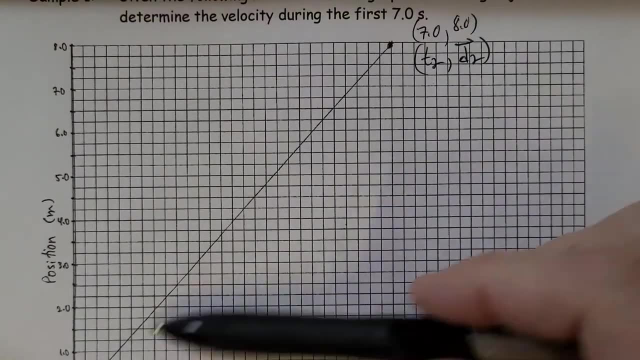 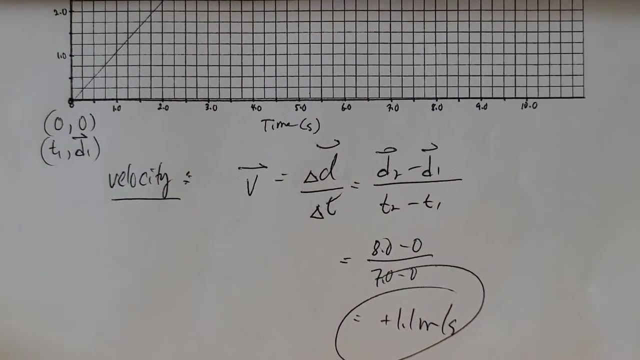 So that will give us plus 1.1 meters per second. So the velocity at any point here, how fast are you going? 1.1 meters per second. 1.1 meters. The straight line, the slope at any two points here is going to be 1.1 meters per second. 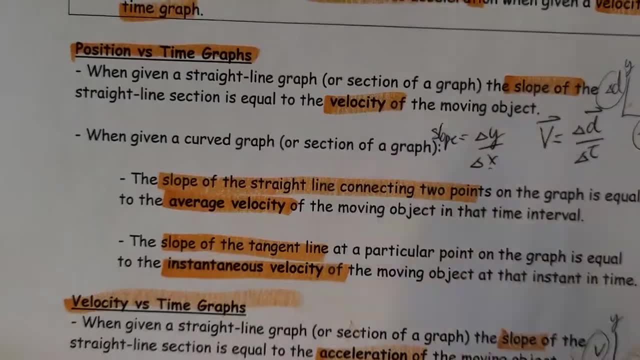 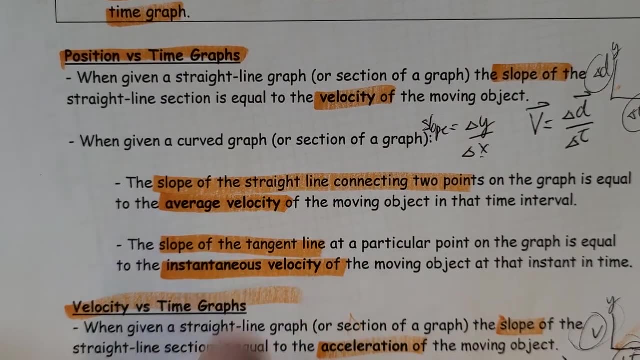 And I'll treat that as being positive. All right, let's take a look at a scenario in which I don't have a straight line graph, but I have a curve graph. I can figure out the average velocity between two points, And I can also figure out the instantaneous velocity between two points. 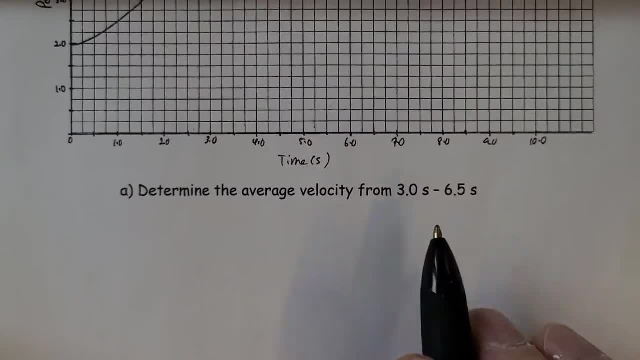 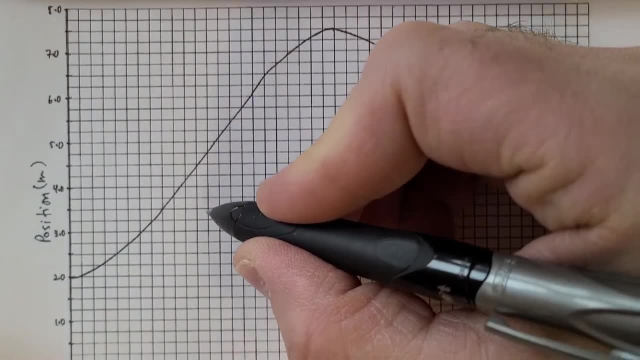 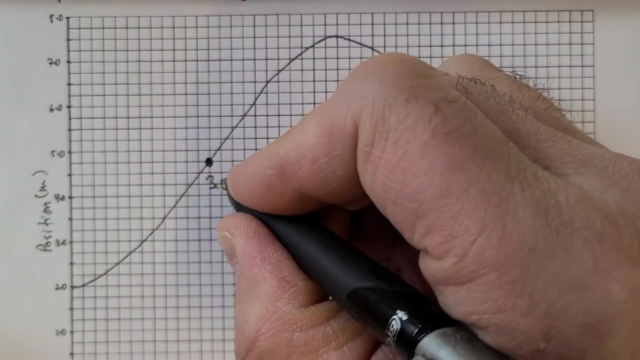 So if I have a scenario like that, what is the velocity? from 3 to 6.5 seconds, So 3.. Let's see, So 3 is right here And that is going to be approximately 3 comma And you can see it's 4.75.. 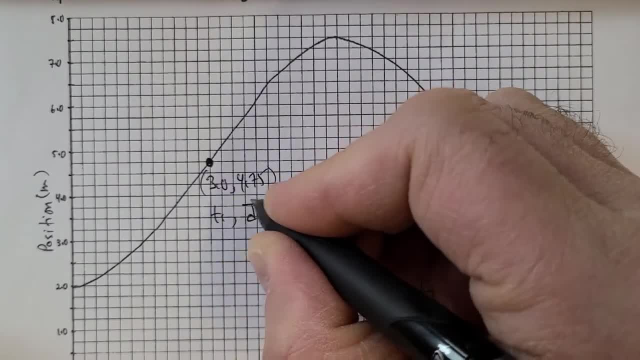 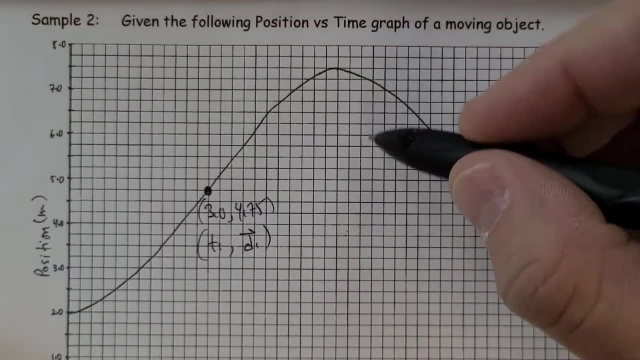 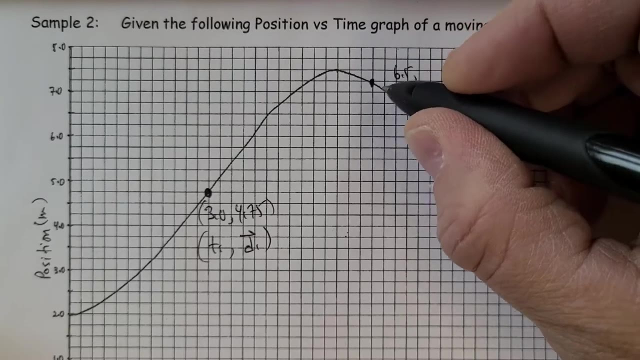 So that's T1, D1.. And then at 6.5.. So right here is 6.7.. So 6.5 is right here in the middle. So around right there. That is approximately So 6.5 comma. 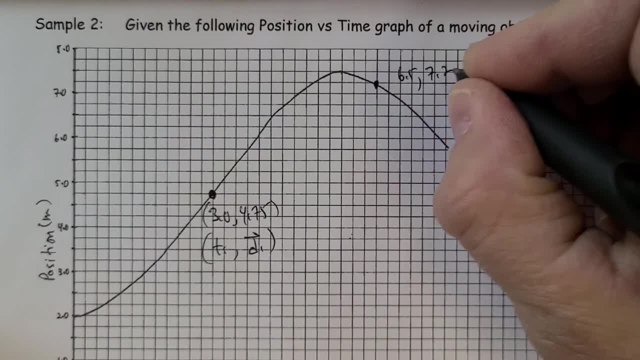 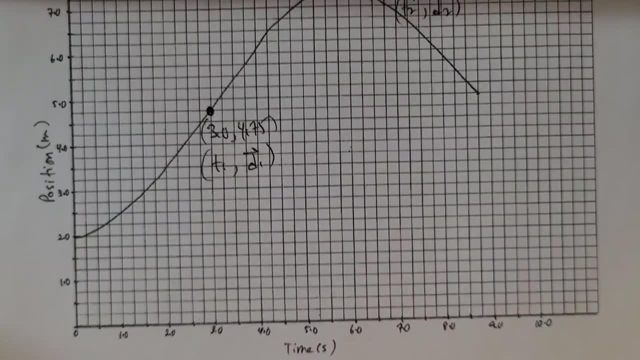 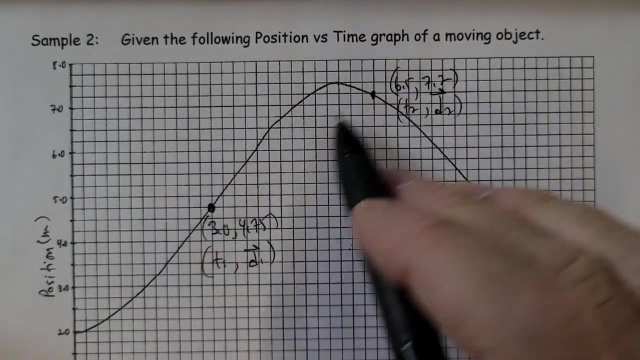 Well, let's see here It's around 7.2, I think. So that's T2, D2.. Not to be confused with R2, D2.. So what I'm really doing there is I am figuring out the slope of the line that's joining those two points. 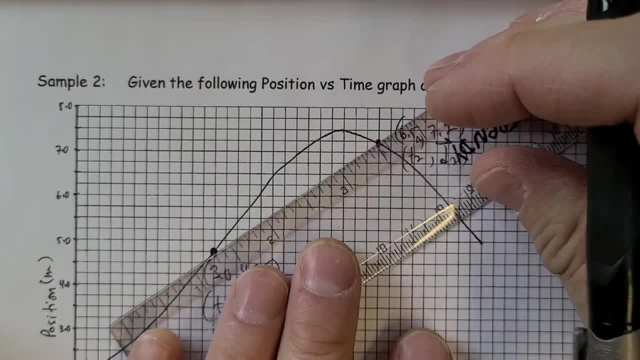 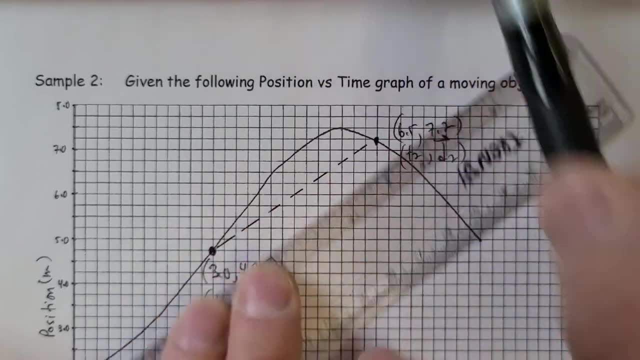 So if I want I could get a ruler here. So basically it's the average velocity would be The slope of a line joining those two points. I'll just write it as dotted so we could see it. So really, what I'm doing is figuring out the slope of a line there. 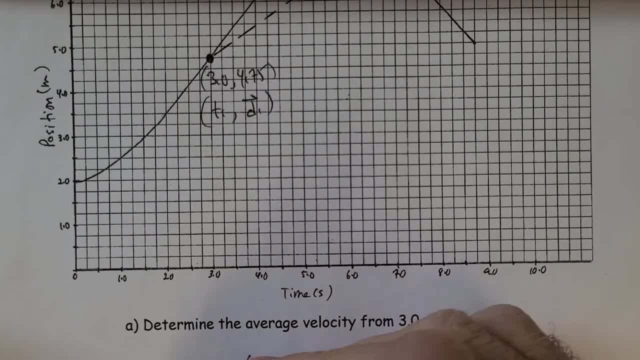 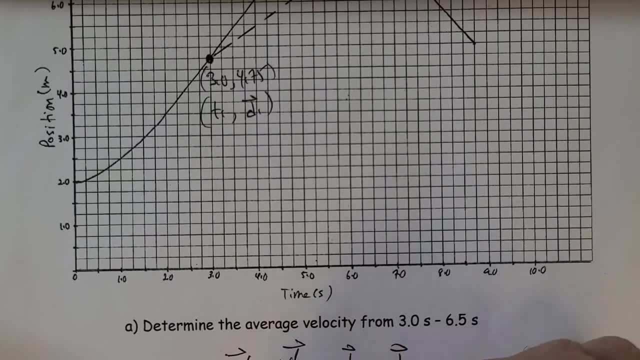 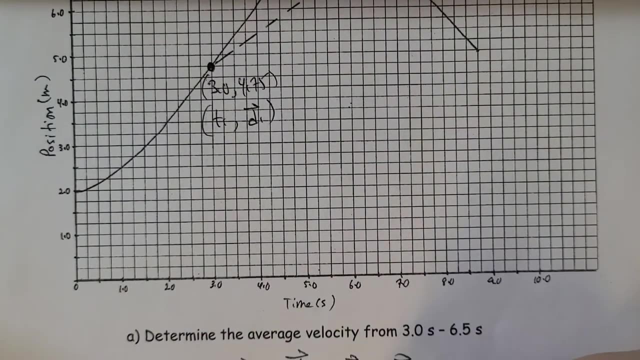 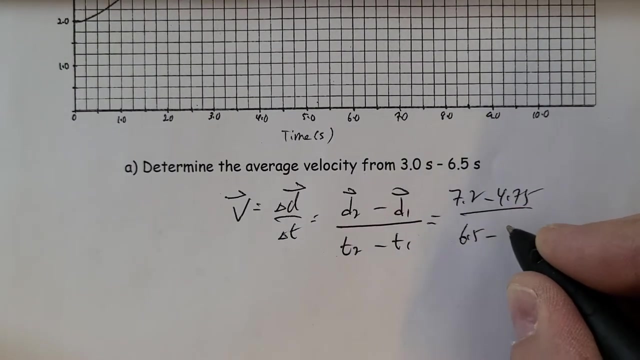 So V is equal to delta D over delta T, In this case D2 minus D1 over T2 minus T1.. So D2 is 7.2 minus 4.75.. And my 2 times 6.5 minus 3.0.. 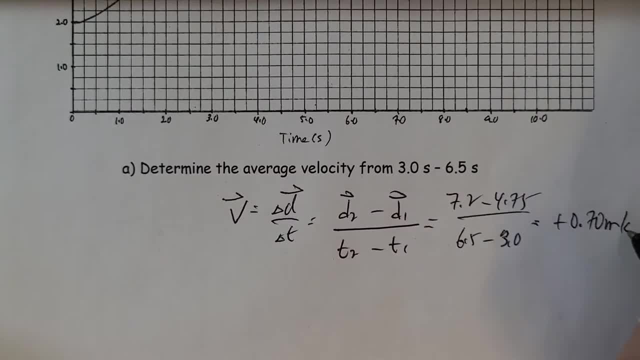 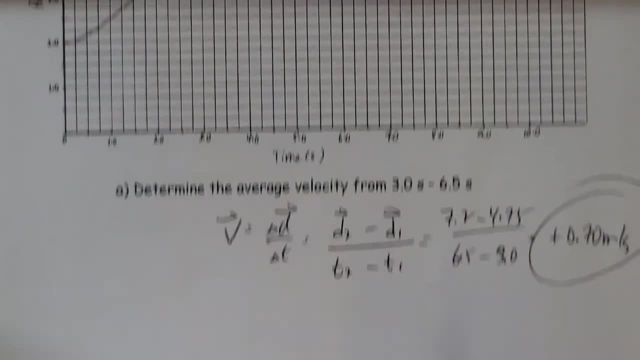 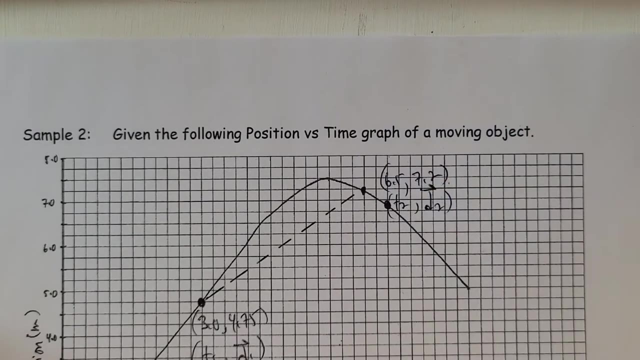 So that's going to give me plus 0.70 meters per second, approximately All right- And instantaneous velocity at 7.. So I want to look at what's happening at exactly. Oh, I have tons of writing on there. That's too bad. 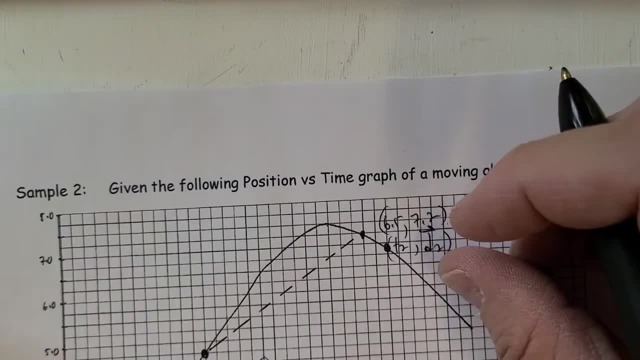 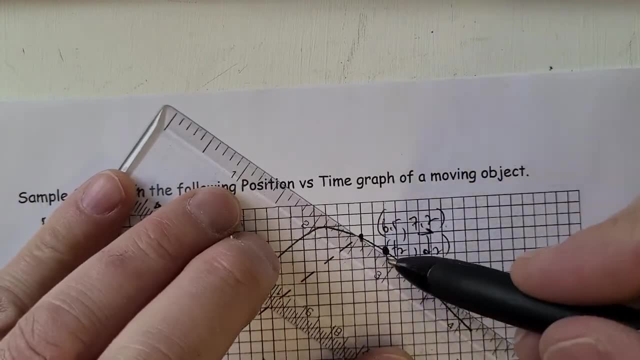 Now, for our intent and purpose, what we can do to figure out a 10.. We want to figure out the slope of a 10.. We want to figure out the slope of a tangent line, So to make a tangent. like you can see, that the slope in this area here is kind of doing what my ruler is showing. 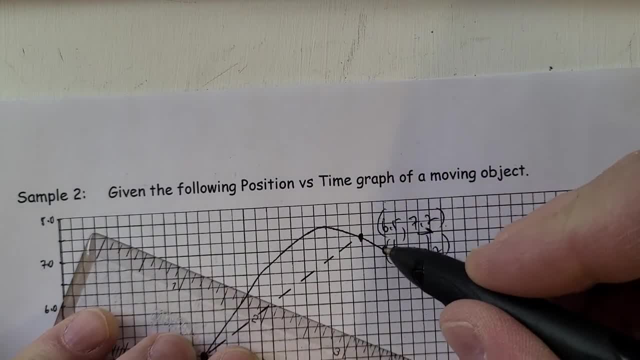 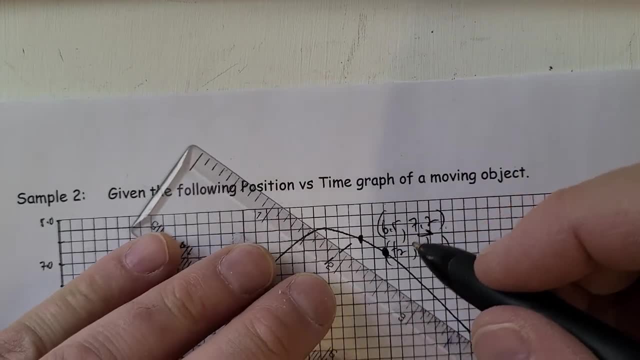 Now, an easy way to figure out the exact slope is to look at the point in question. Now we just simply can't take this point and this point and divide, Because, again, a slope requires two points. So what we can do is we have this point here. 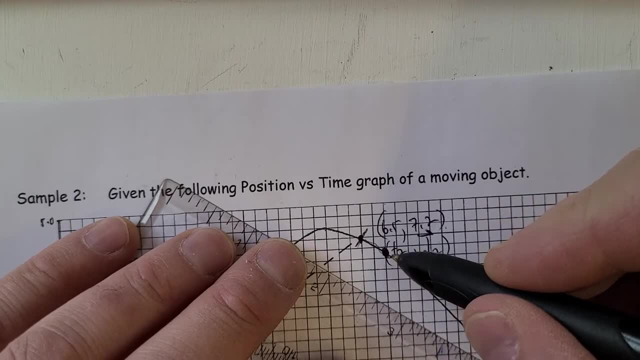 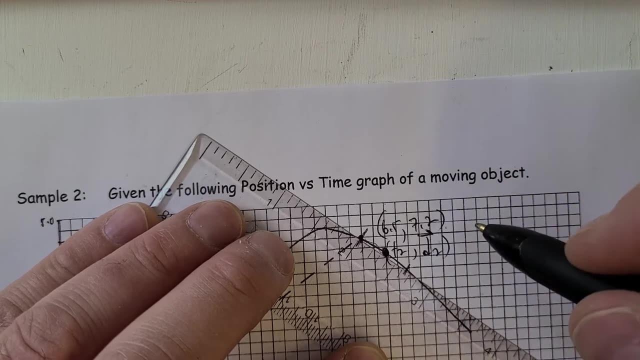 And you can see how far it is away from that. 7 second line. Make an equal point On the opposite side. So I'll have that And take your ruler and match those up So you can see here this will be approximately the slope. 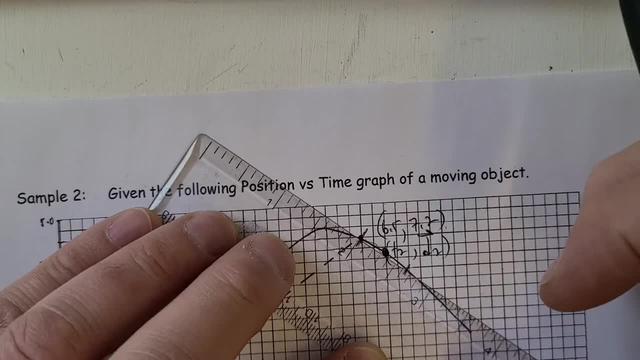 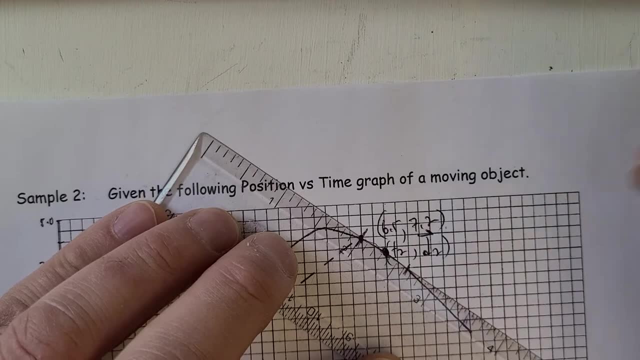 But what I have to do is move my ruler up. so it just is at that point. So, keeping the slope of my ruler as is, move it up. so we just see that point, There we go, And then that would be my tangent line. 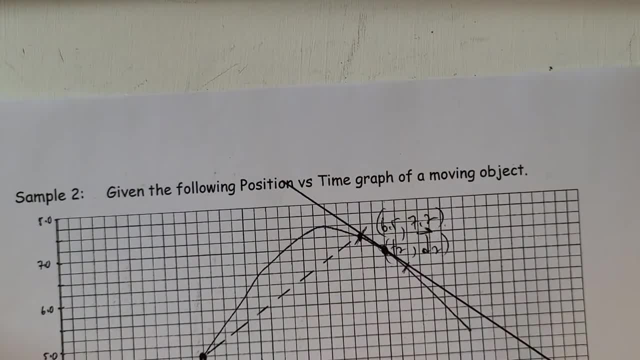 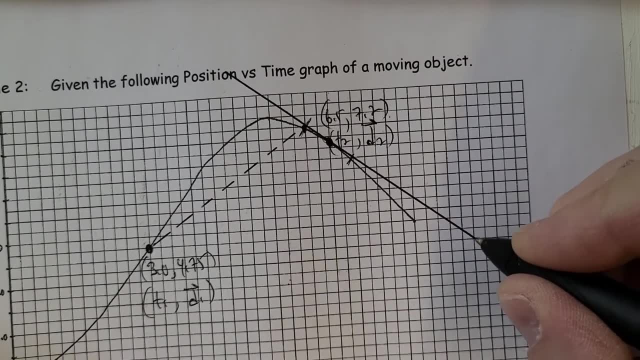 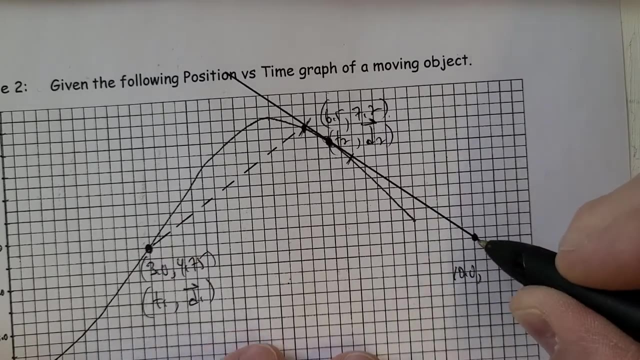 And then all I need to do is pick two points That fall on that tangent line. What to look for is look for two points that kind of fall That are going to be easy to read, Like you can see here. this one here is at 10, 4.5.. 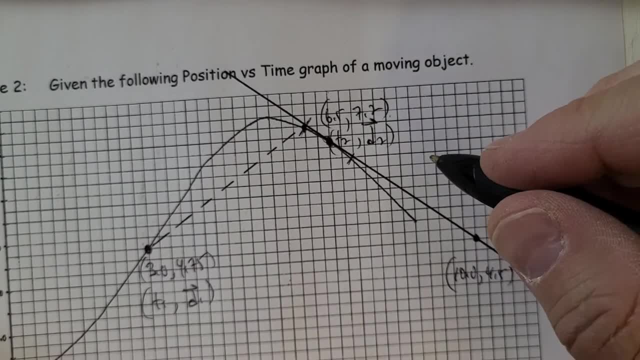 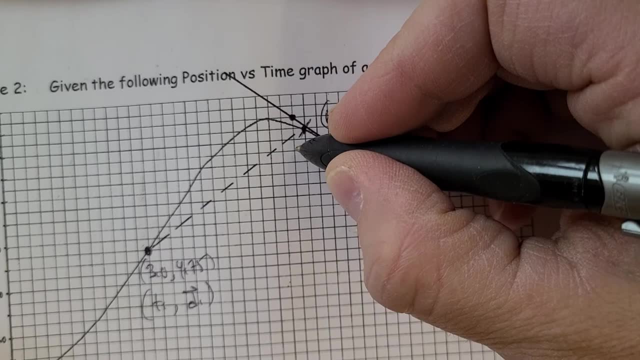 So yours will likely be a little bit different than mine, Because you likely drew your tangent line slightly different. And this point right here is at a crosshairs too, where two lines meet, So it's at 6., 6.25 and 7.5. 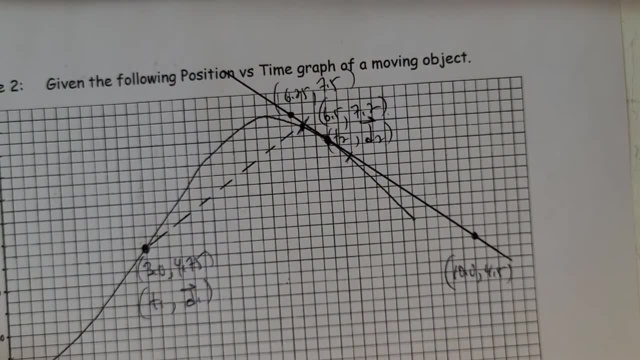 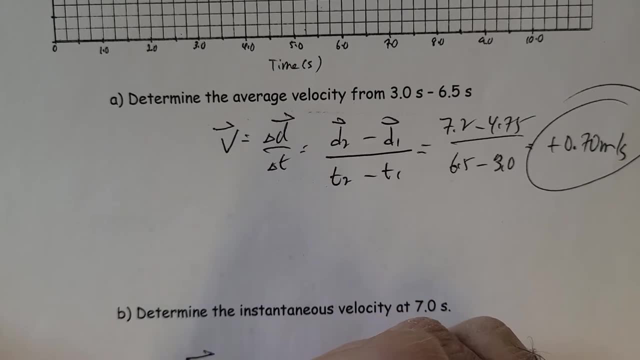 So those would be the points that I am going to use, And again, yours will be different likely, But we should get similar to the same answer. So V is equal to change in D over change in T, D2 minus D1 over T2 minus T1.. 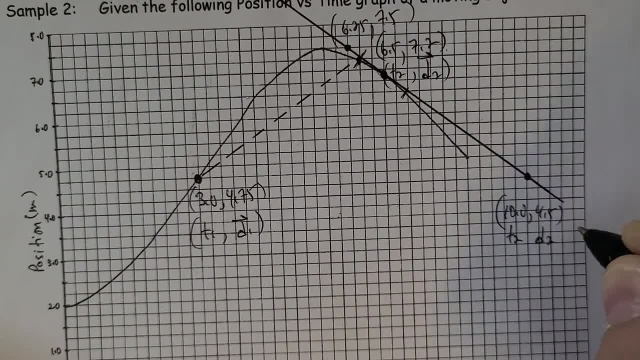 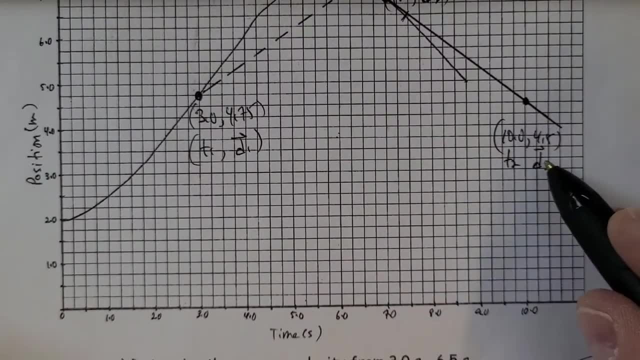 So my let's see here. So this is going to be T2, D2 for this particular Question and this one is T1, D1 from this particular question. So D2 is 4.5 minus my D1 is 7.5.. 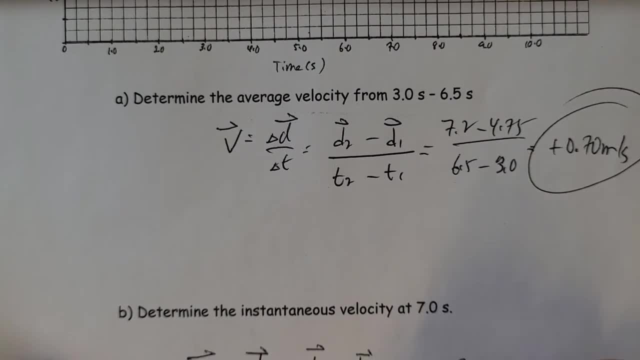 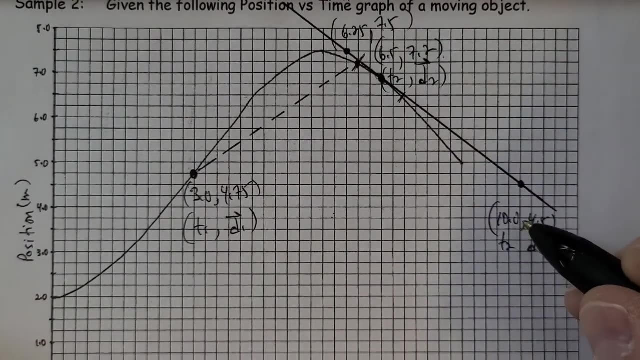 So 4.5 minus 7.5.. Okay, So that's what I get for mine Now, yours will likely be a little bit different, Remember that's okay. And then 10 minus 6.25,, 10 minus 6 point. 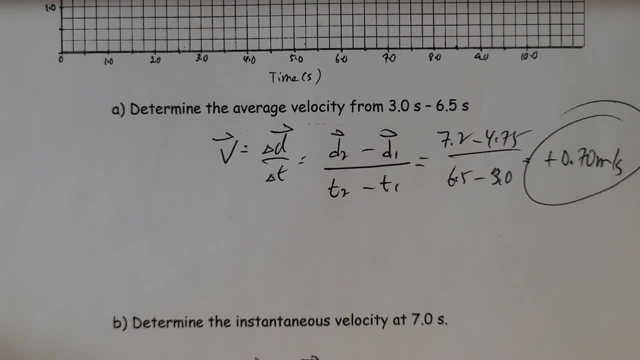 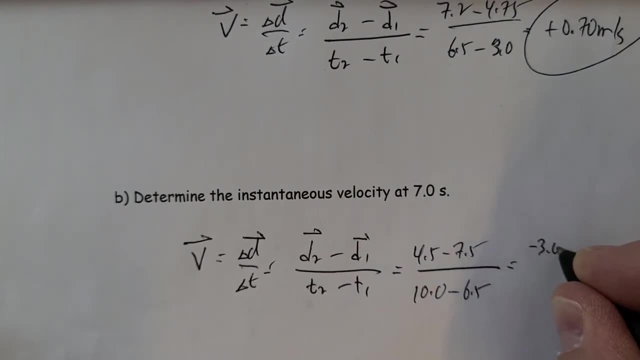 Oops, six point. Well, it's a 6.5, I guess. All right, so we're figuring that out. I'm going to get, uh, so negative three on top and then on the bottom I'm going to get 3.5.. 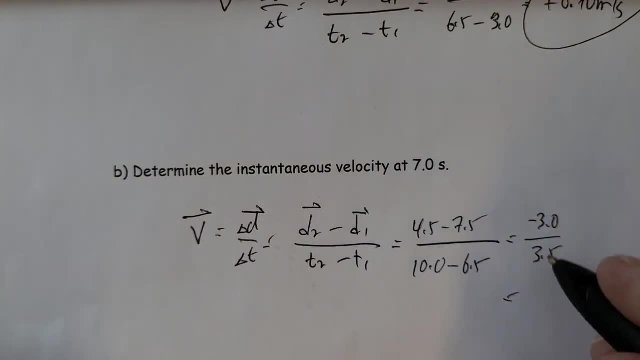 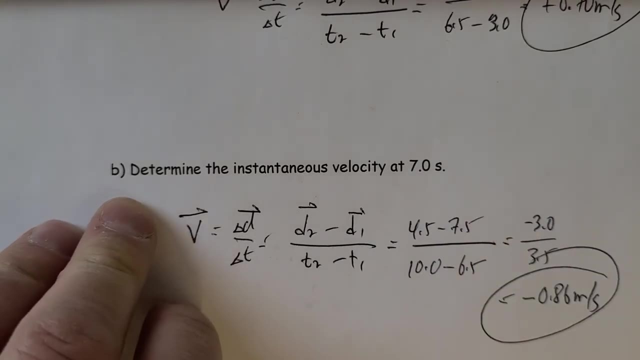 So negative three divided by 3.5 is going to give me negative, which makes sense: Negative 0.86 meters per second approximately. So you can see, yes, it's a negative slope and it's going to be less than one. 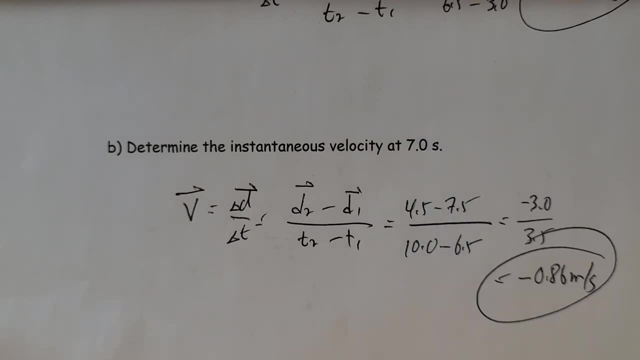 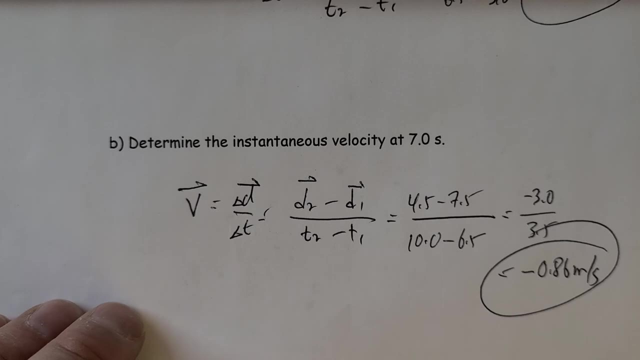 So Take a look at yours. You should get a slope that's a little bit less than one and, of course, negative, And uh, that's what you should get, So something very similar. Okay, Think what I'll do is I'll stop there and, uh, we'll look at part two and look at the final example.